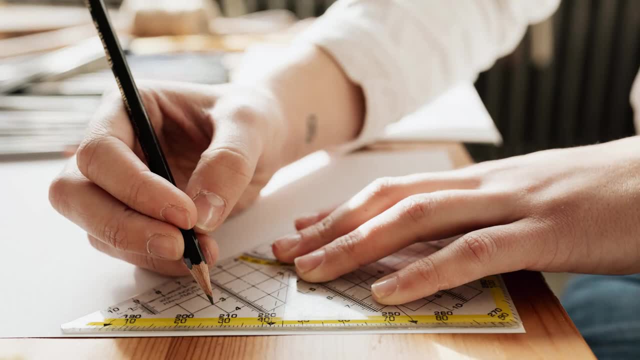 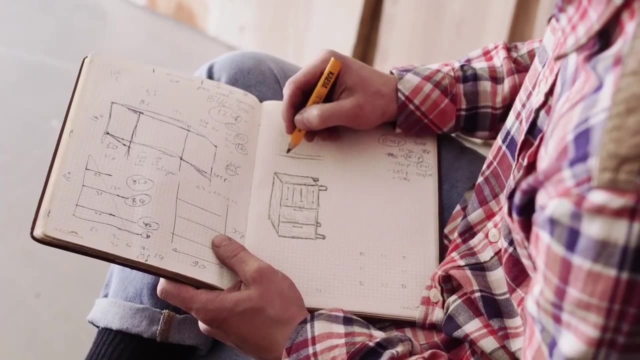 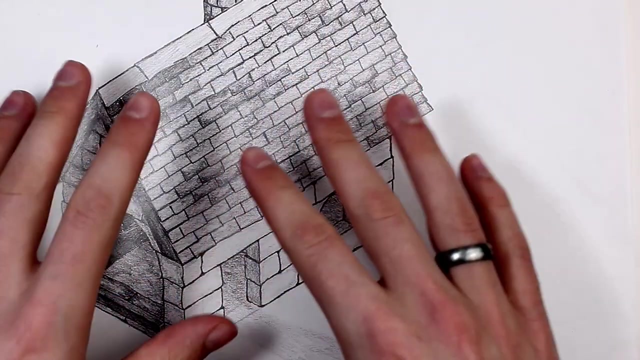 that is especially suited for design. It can be used to draw precise, functional drawings to explain how something works or how something is put together, Or it can be done freehand for quick, accurate sketches that allow the designer to get their ideas down onto paper really rapidly. 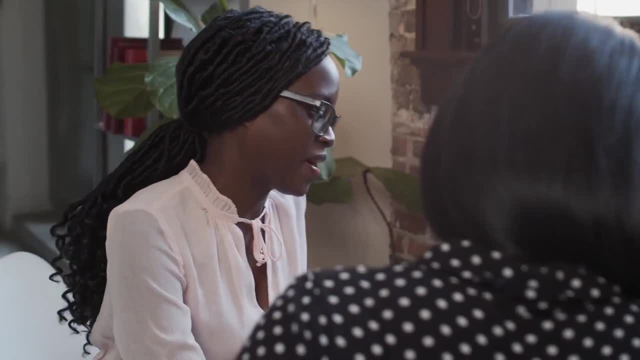 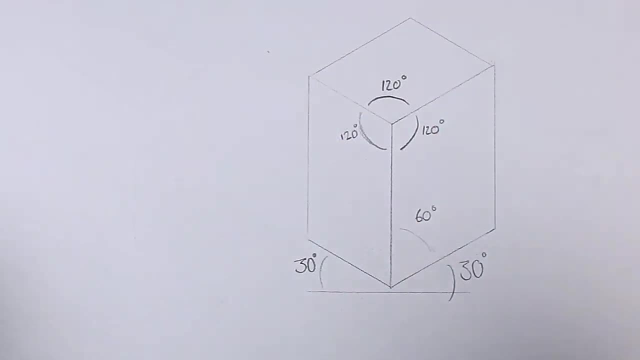 These freehand drawings are often accurate enough for a designer to show to clients in the early stages of a design to work out if the design is developing the way the client wants it to. Everything in isometric drawing comes in multiples of three. So in isometric drawing we 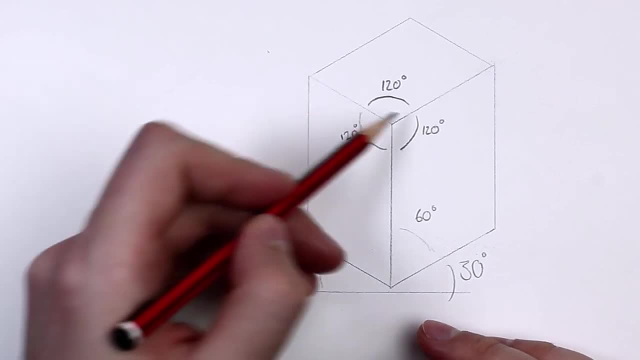 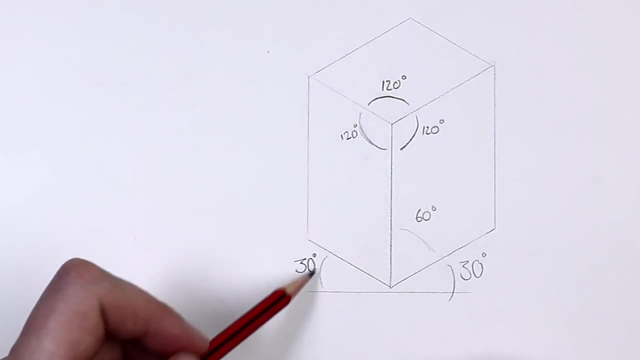 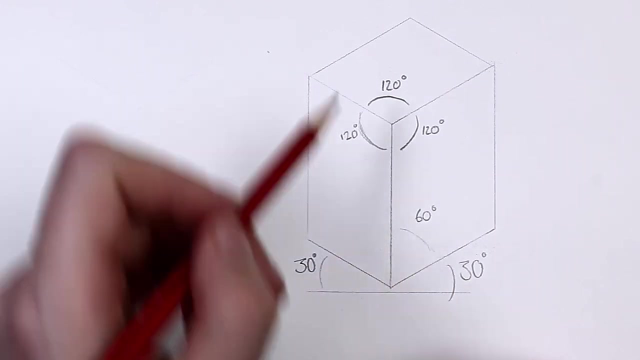 have three directions of line. we have vertical and we have two different diagonals And those diagonals are the same all the way through the drawing. Those diagonals are at 30 degrees- another multiple of three from a horizontal line, or at 60 degrees when they're close together. 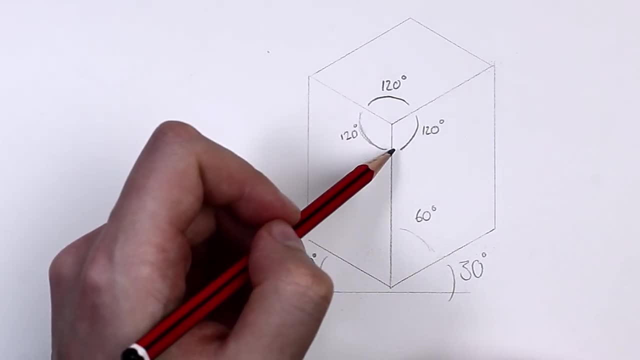 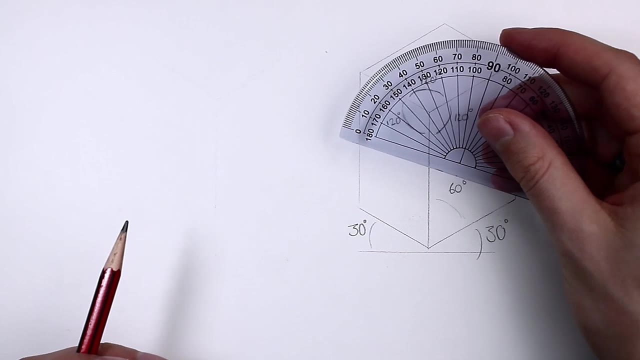 or at 120 degrees when they're a bit further apart. So that's, everything is in these multiples of three. So if you wanted to be really accurate with your drawing, you could get out a protractor and you could measure each of the three. And if you wanted to be really accurate with your drawing, 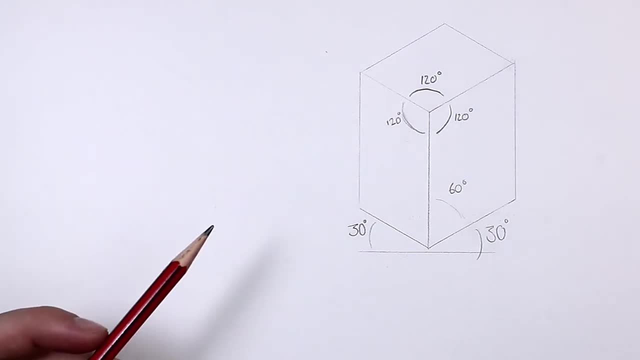 you could get out a protractor and you could measure each of the three. And if you wanted to be really accurate with your drawing, you could get out a protractor and you could measure each of these angles perfectly. Or you could get yourself one of these, those random triangles from your math sets. 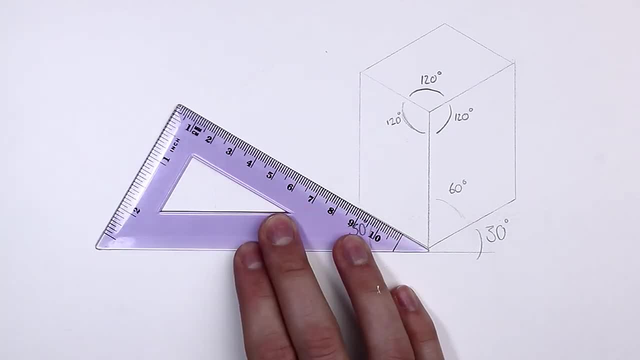 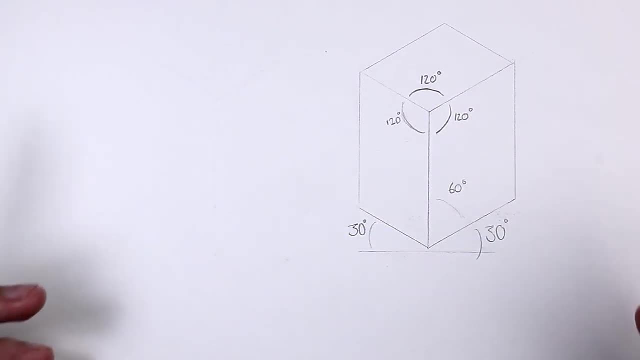 it's called a set square, and that will give you your 30 degree angles or your 90 degree angles really, really easily. If, like me, however, you're using isometric drawing just to sketch out some ideas, you can do this by eye as well. The easiest way I find to do this is 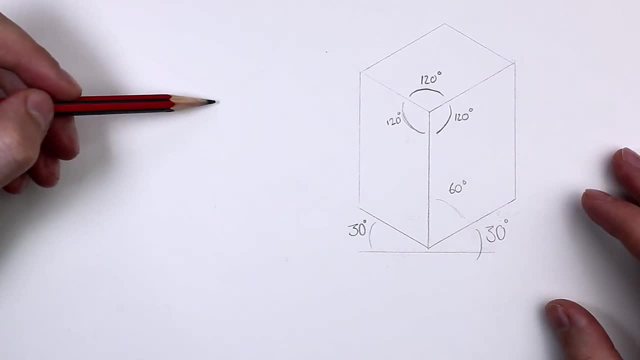 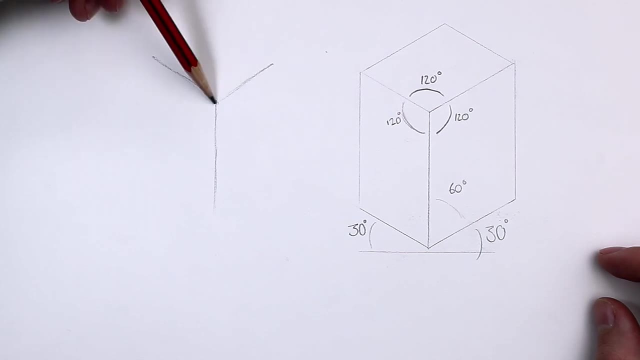 to start off with a letter Y, because that shape gives me all of these lines And it's quite easy to do by eye, because you can very quickly tell if it's off, because these angles will look quite different from each other. So as long as these. 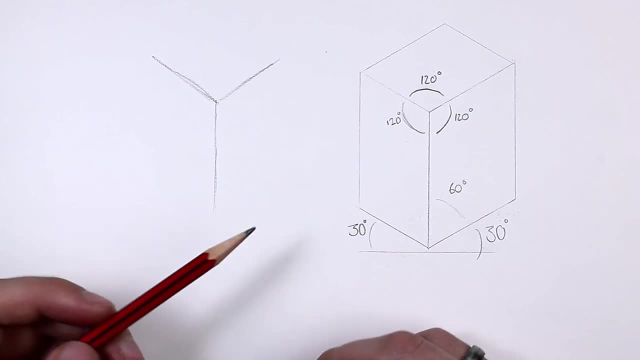 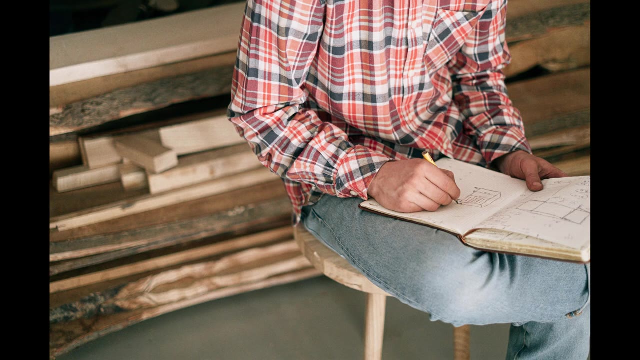 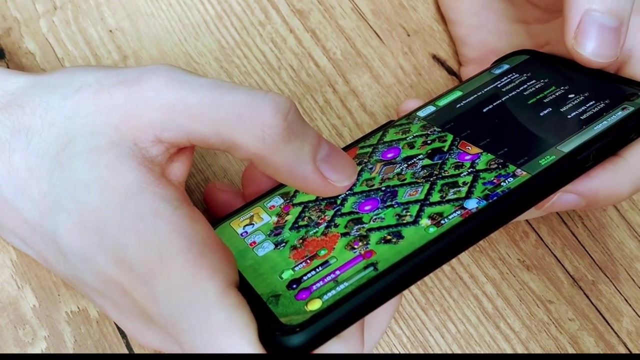 angles look roughly the same. you've got it roughly accurate Now. isometric drawing or isometric projection is now used in a variety of other settings, from exploded drawings in Flatpak Furniture Instructions to mobile game design, Because isometric drawings always look like they're being viewed from that one corner. one of the benefits is that, unlike perspective,